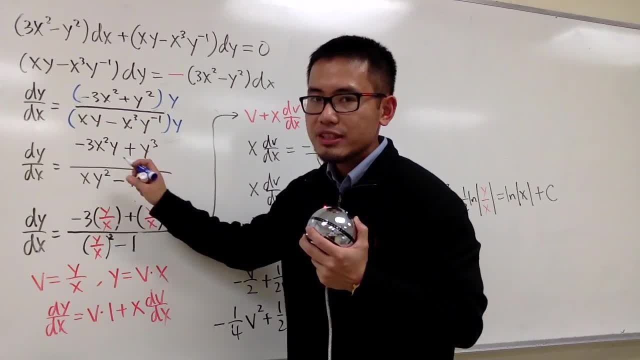 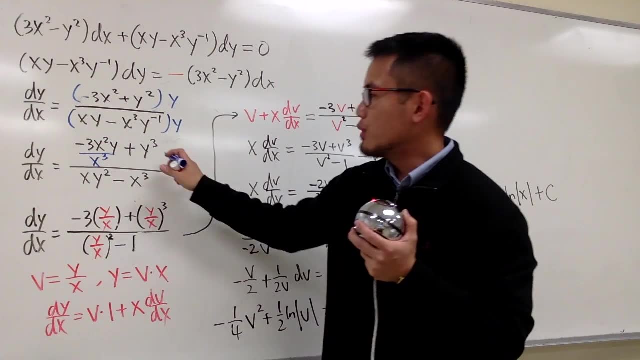 And the idea, the strategy, is that let's go ahead, divide everything by x to the third power. So, right here, let me just divide this term by x to the third power, and then we do the same for the rest, Right here, divide everything by x to the third power. 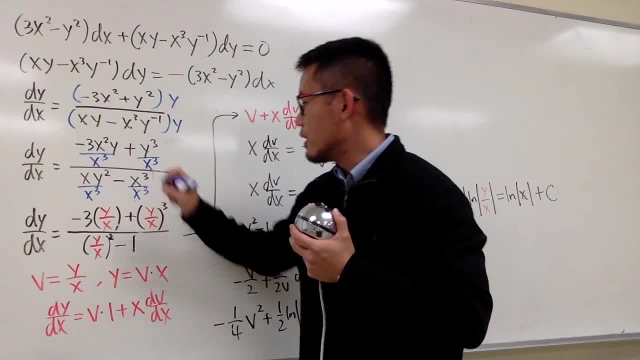 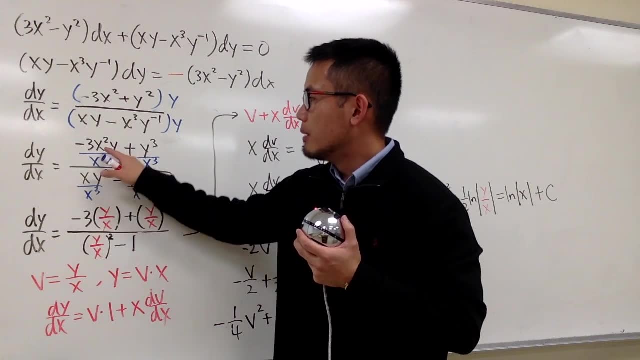 Do the same right here. Divide this by x to the third power- third power as well, okay. and then you will see here we have negative 3 right here. but this is x squared over x to the third power. that means we have an x in the denominator. we still have the y. 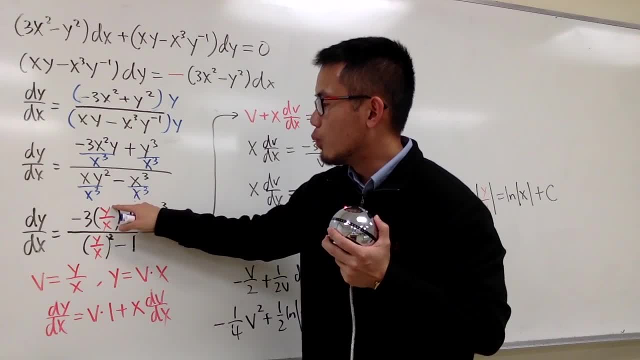 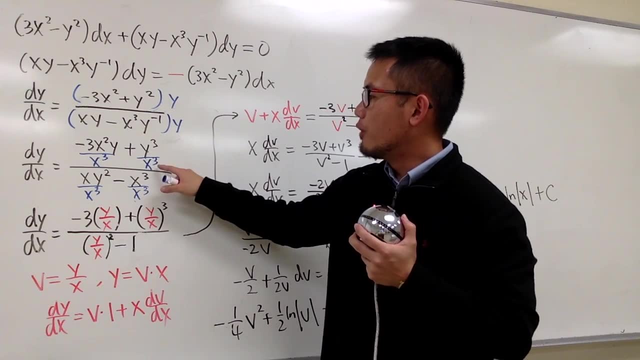 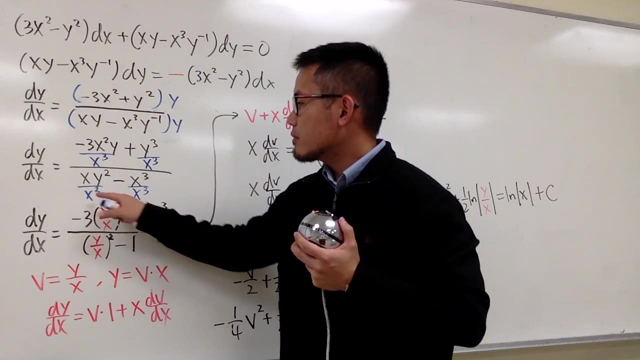 on the top though. so that means we will have this right here to be y over x, with the negative 3 in the front, and then for this term, you see, we add y to the third power over x to the third power. we can write this y over x first and then raise to the third power and then, for this, x over x to the. 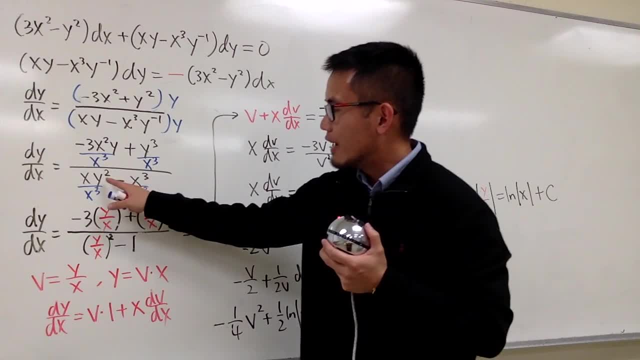 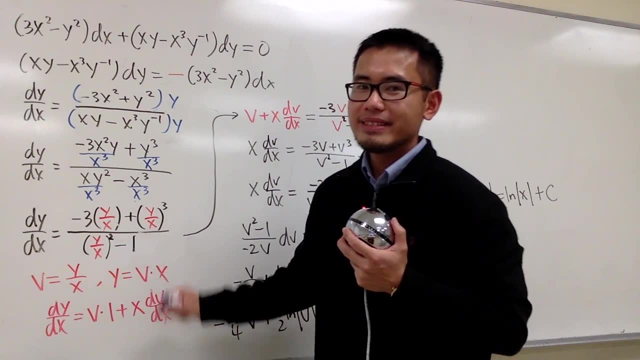 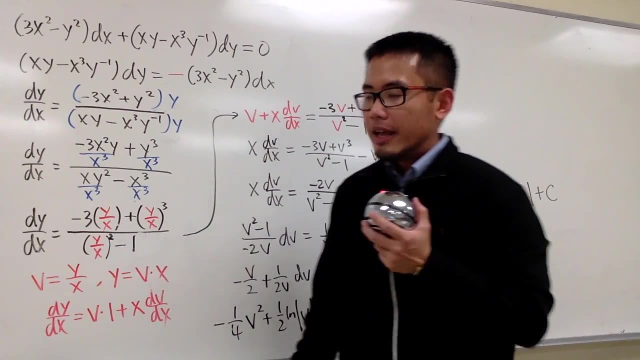 third power. it's x squared in the denominator, but then we have y squared on the top. so we can rewrite this as y over x first and then square right at the end. we'll have a minus, and then x to the third power over x to the third power is just 1. so minus 1 right here and now. you see this right here we. 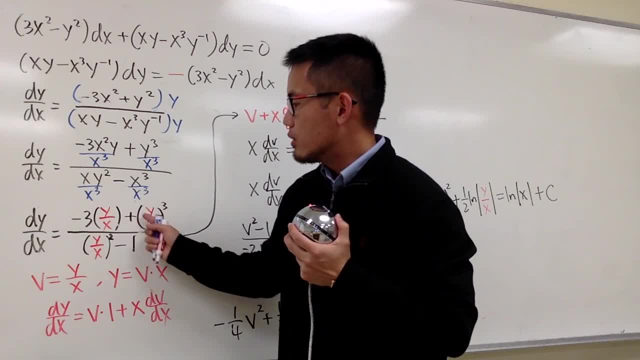 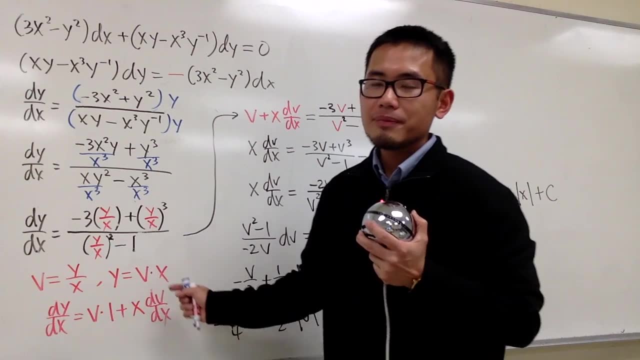 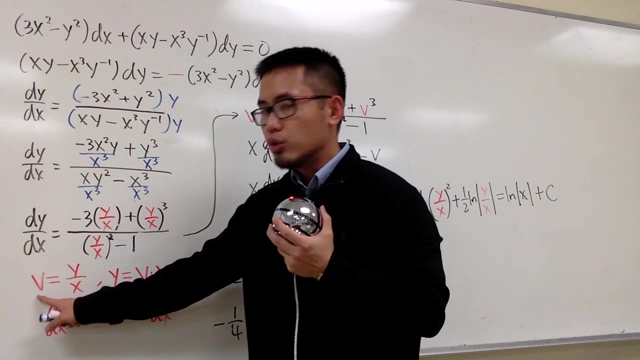 were able to rewrite the right hand side into an expression in terms of just y over x. y over x has to be together like this, right. if this is a situation, we can try the following: this is the substitution that we're going to do. we are going to pick another variable and usually you use v. we let v equals to the input, which is y. 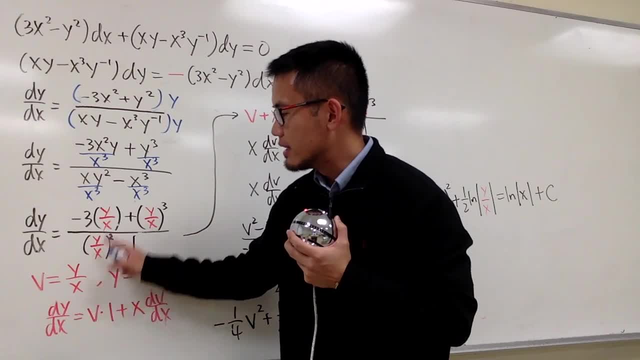 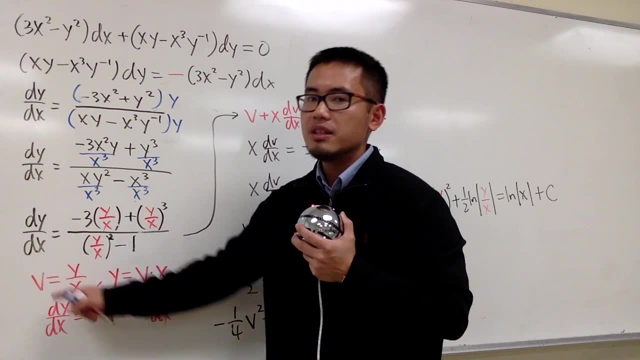 over x. so we let: v is equal to y over x, the input all right. and then the idea is that we have to also get dy, dx, y, dx, y, dx in terms of dv, dx, and perhaps let's just go ahead: multiply x on both sides. that means y is equal to. 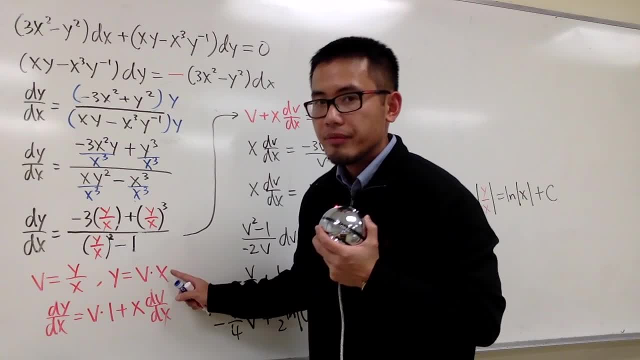 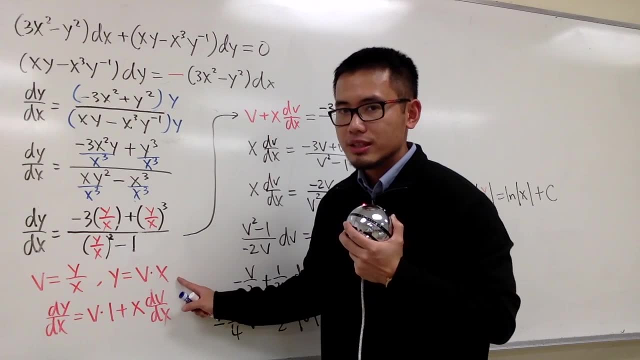 v times x. and then let's look at this, differentiate both sides. the derivative of y is just dy, dx, but on the right hand side we have a product of two things. right, so we are going to use the product rule. so we keep the first and multiply by the derivative of x, which is 1, and then we add it. 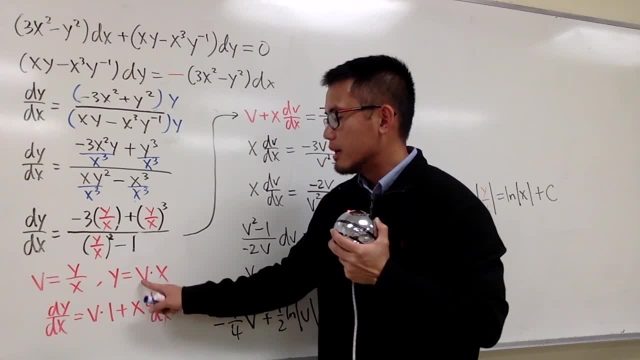 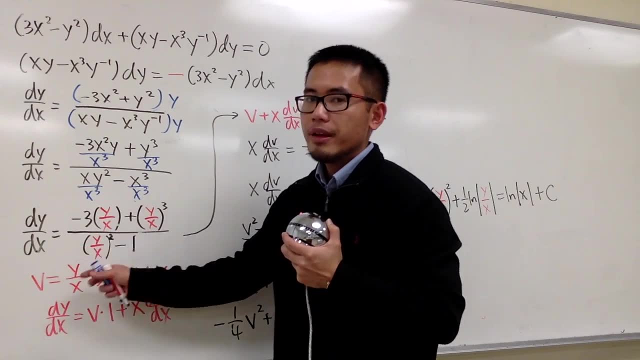 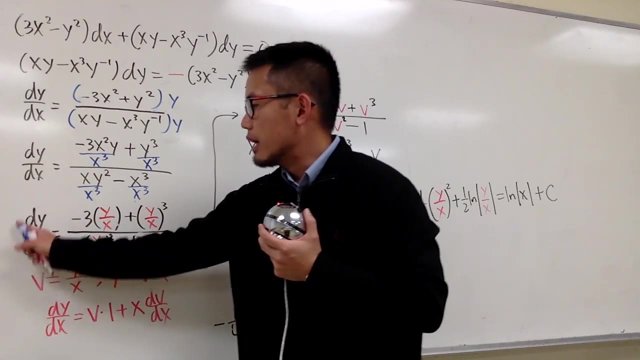 with the second function, which is x, and we multiply by the derivative of b, which is the final function, y becomes x and we multiply to x, also keep multiplying, and we add one equal to y to get the inner objection value of 2x, dy, dx and x, dv, dx. and now we are going to use these. 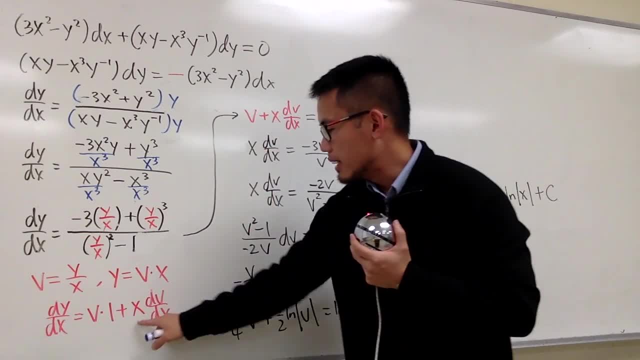 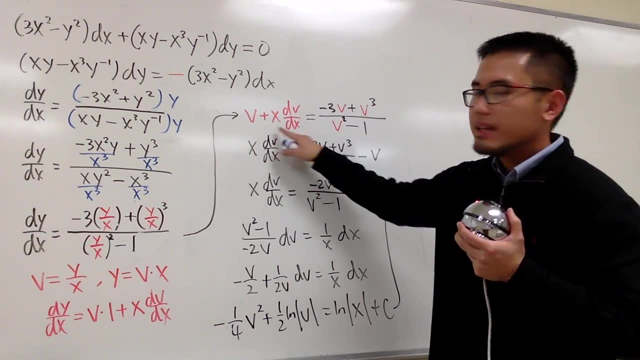 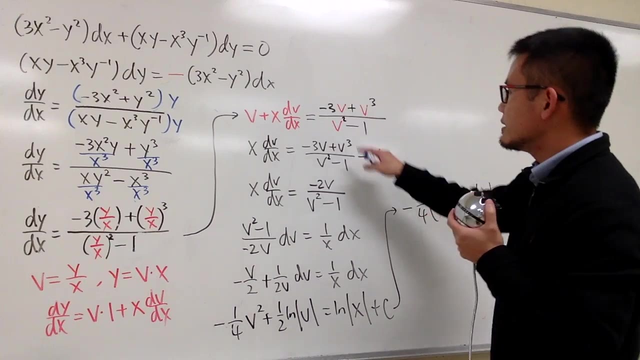 ingredients plug into here, and then we write this differential equation in terms of v, dpdx and also dx, And then this is equal to: I will change all the input instead of y, of x into phi, So on the right-hand side we will have negative 3 phi right, And then plus phi to the third power. 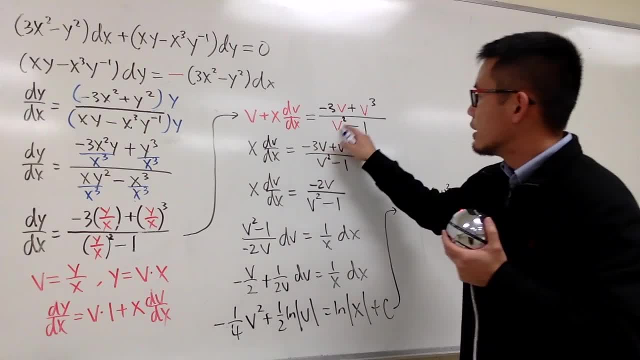 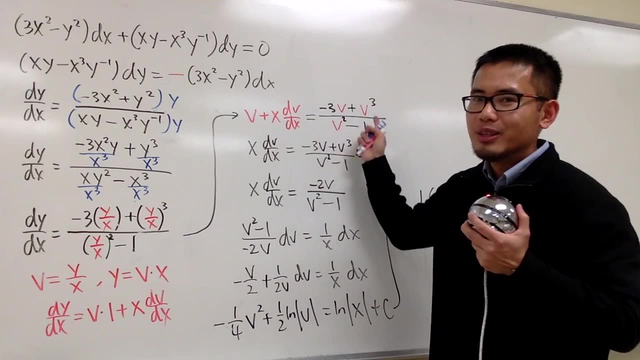 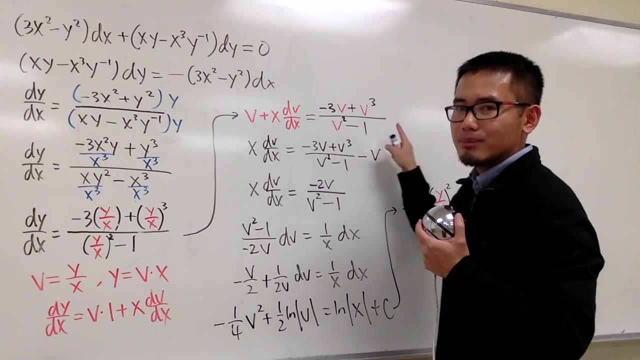 and then over phi squared, and then we have the minus 1.. And now let me tell you, this is guaranteed to be separable. So you see this right, here is phi plus this term. So let's go ahead: minus phi on both sides, And this is what we have, isn't it? Well, on the right-hand side, 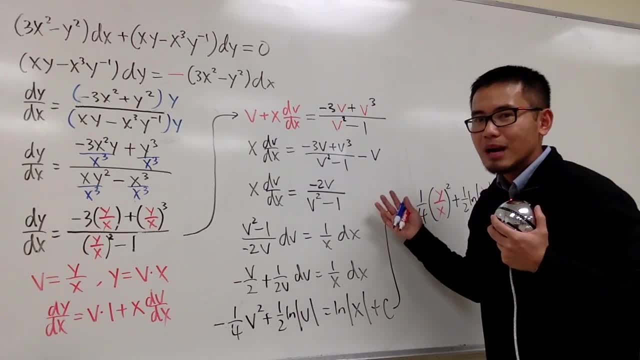 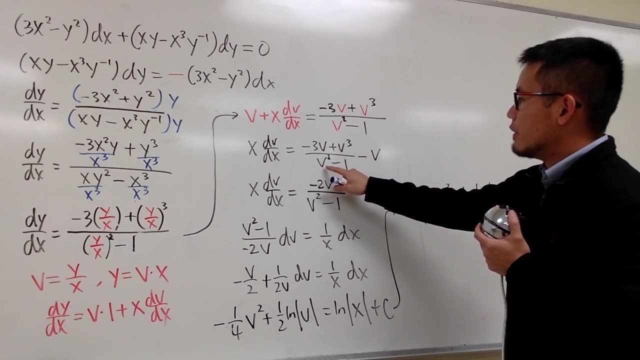 we are subtracting fraction with phi. Let's just get a common denominator so we can combine fraction and see what do we get on there. So the common denominator will just be phi squared minus 1.. So right here, let me just multiply the bottom and the top by phi squared minus 1.. So I'll do. 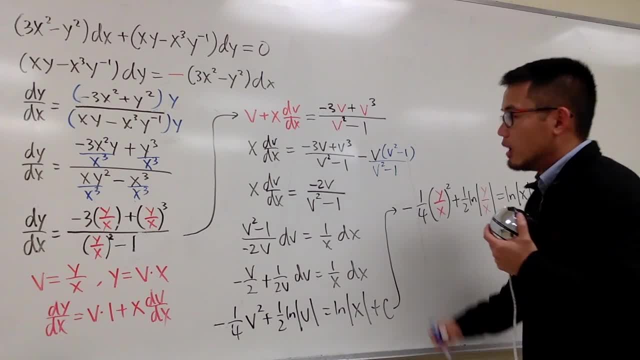 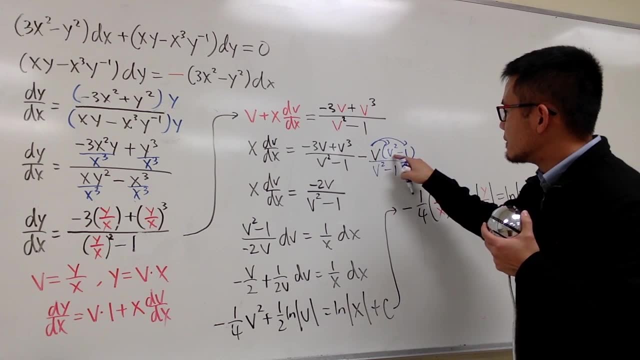 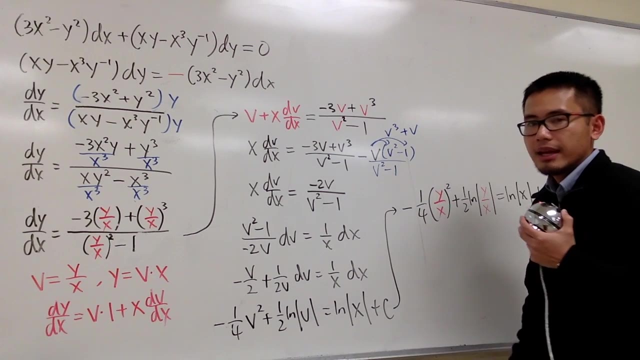 the same right here. phi squared minus 1.. And let me just distribute this as well, but be sure you account for the negative sign as well. Negative phi times phi squared is phi to the third power. Negative phi times negative: 1 is plus phi. And then you see positive phi to the third. 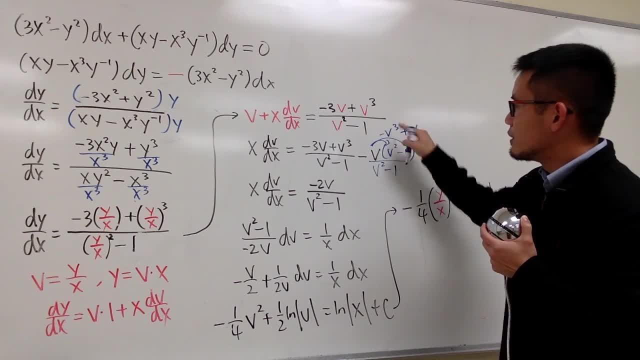 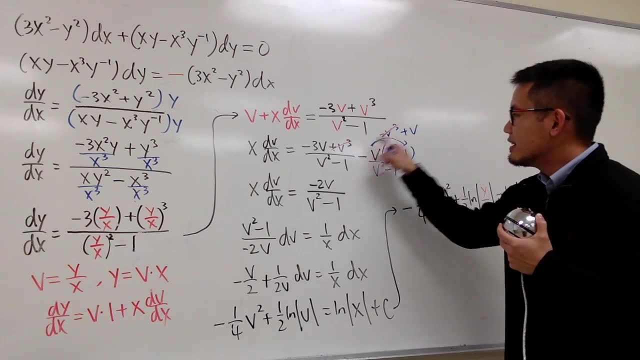 power and this is technically a negative right. Negative phi to the third power. These two cancel out, right. This is negative phi times phi to the third power is negative phi to the third power. This and that cancel out And then negative. 3 phi negative. negative was plus right Negative. 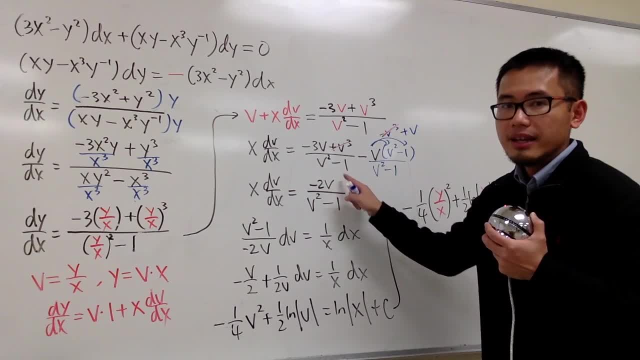 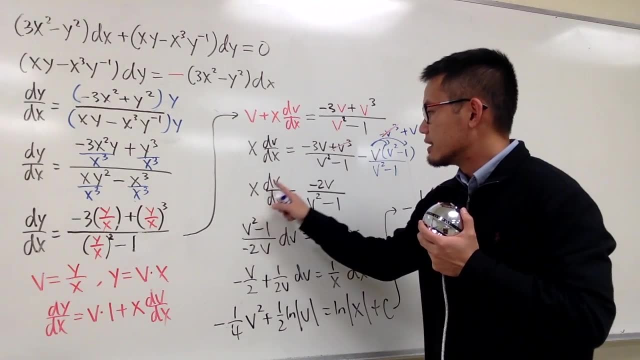 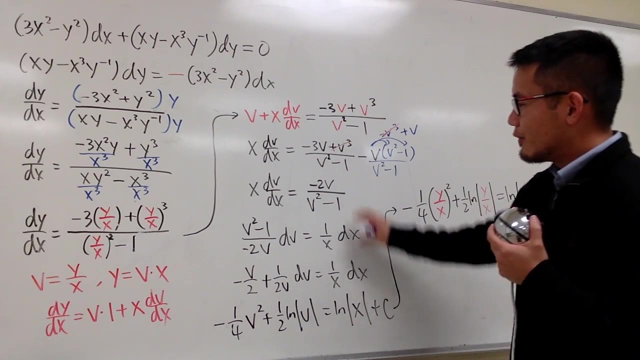 3 phi plus phi becomes negative 2 phi, And this is what we have on the top And the denominator states the same. So now we have x times d phi. dx is equal to negative 2 phi over phi squared minus 1.. So of course I can just multiply both sides by the reciprocal, So we have phi squared. 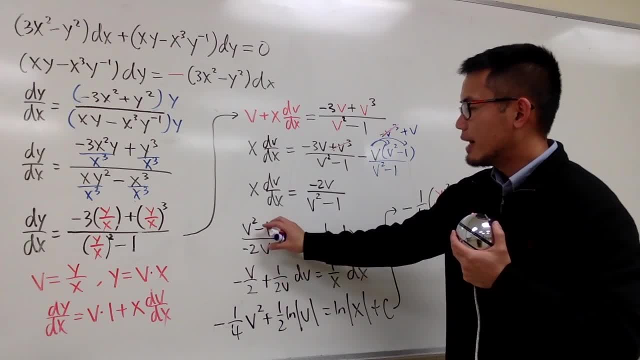 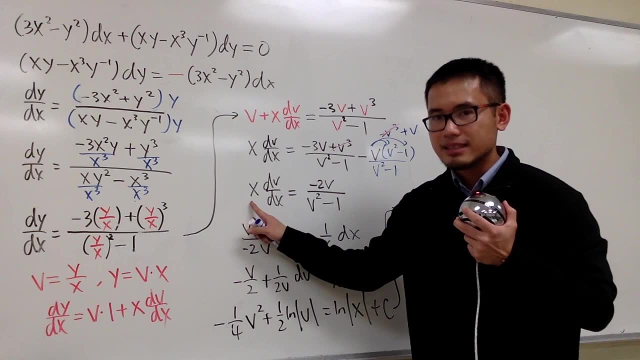 minus 1 over negative 2 phi right And let's keep the d phi on the left-hand side And let's multiply dx on both sides. In the meantime, let's divide x on both sides, So this x becomes 1 over x. 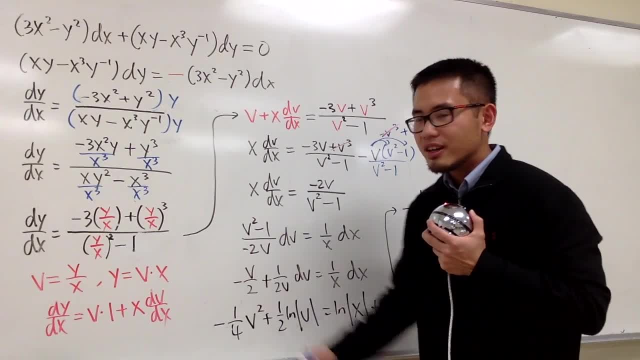 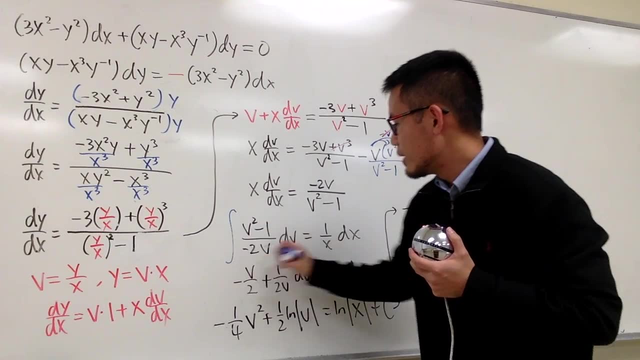 on the right-hand side. now All the phi's and d phi's are together, and all the x and the dx are together, So of course this will separate the variable And then we can just go ahead and integrate both sides. On the left-hand side: to integrate this, let's split it. 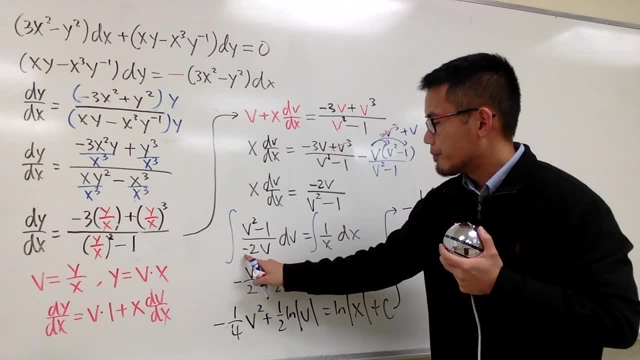 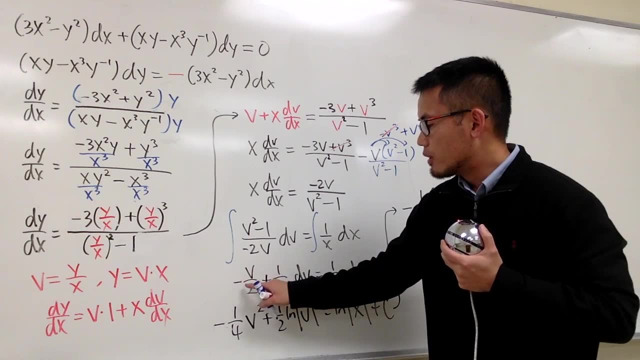 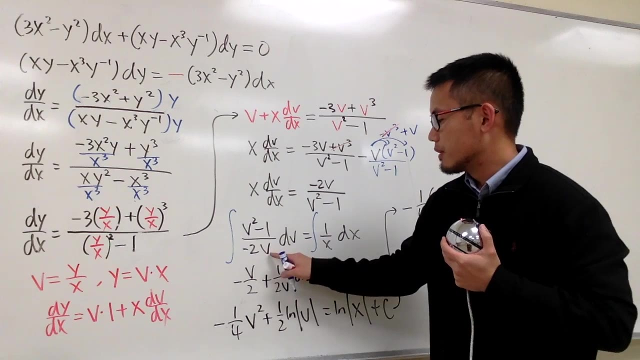 into fractions. So all I did was phi squared over negative 2 phi, But then phi squared over this. phi is just phi on the top right, So we have phi over well, negative phi over 2, like this. And secondly, we have negative 1 over negative 2 phi, So that's plus Negative. 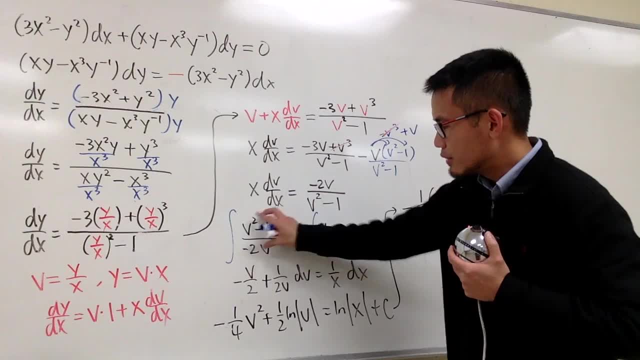 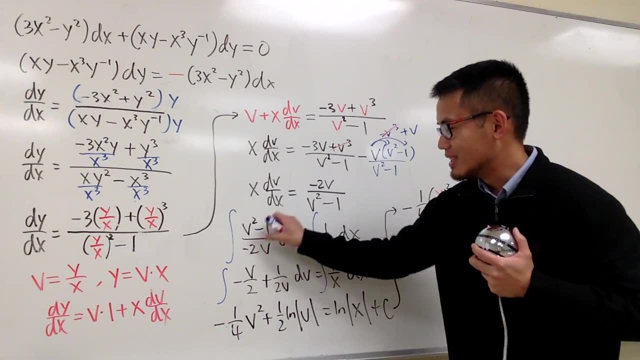 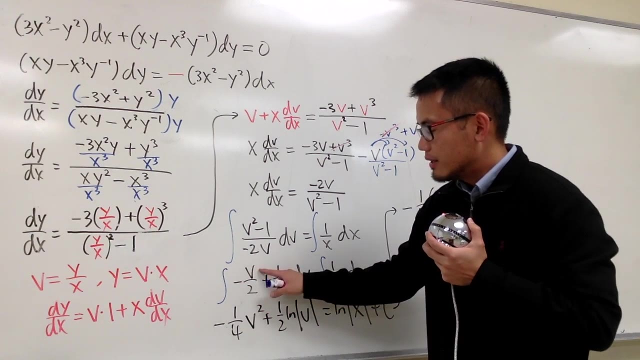 negative becomes plus 1 over 2, phi, like that. So I have to separate the fraction, like this. And then let's talk about integration. right, here I haven't done any integration yet, It's just separate, Split it into fractions, All right. Anyways, here, this is phi, right, Phi to the first. 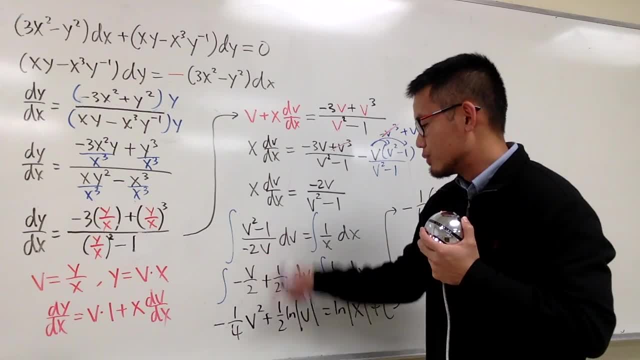 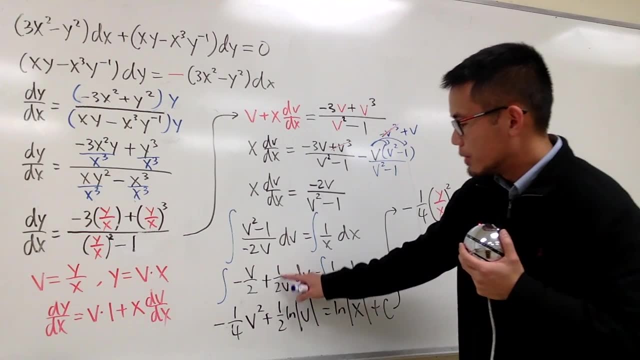 power. So we're going to add 1 to the power and then divide it by 2, right, So we have negative 1 over 4 in the front and then phi squared, And then let's keep the 1 half down. 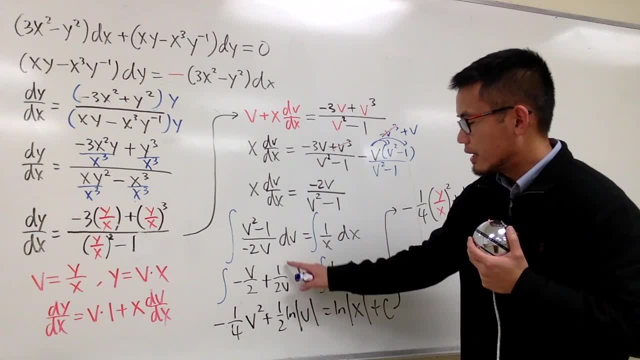 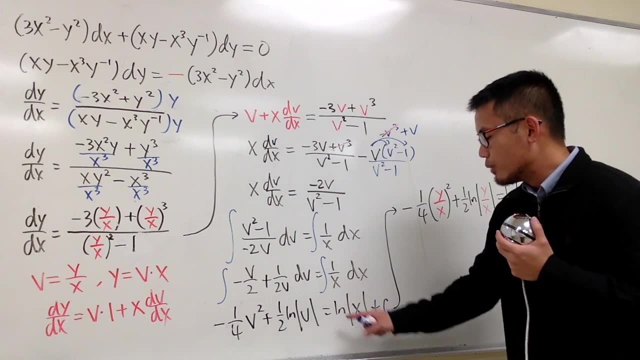 first- because this is just, you know- write down the 1 half, And then the integral of 1 over phi is just ln absolute for your phi, And then this is equal to ln absolute for u of x. right, That's the integral of this. And then we put the plus c on the right-hand. 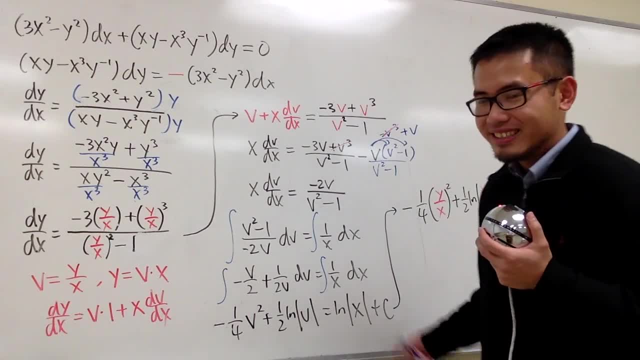 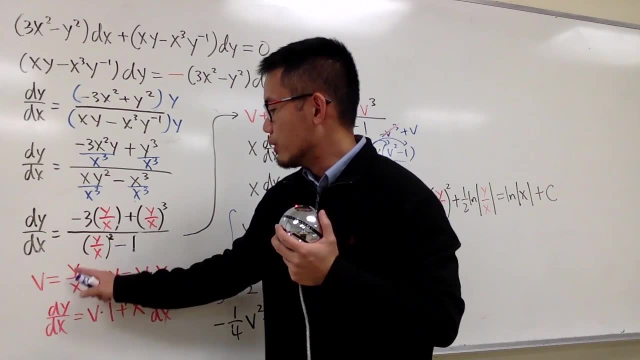 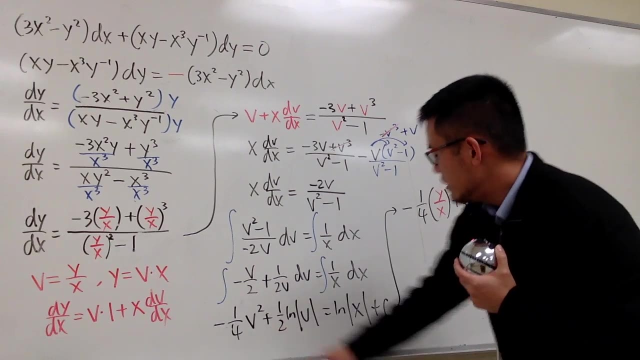 side. All right, So this is pretty much. it, isn't it At the very end, what is phi? Well, refer back to this. Phi is equal to y over x, So I'm just going to rewrite everything back. wherever I see phi, I will put it down as y over x. So I have to do that right here. 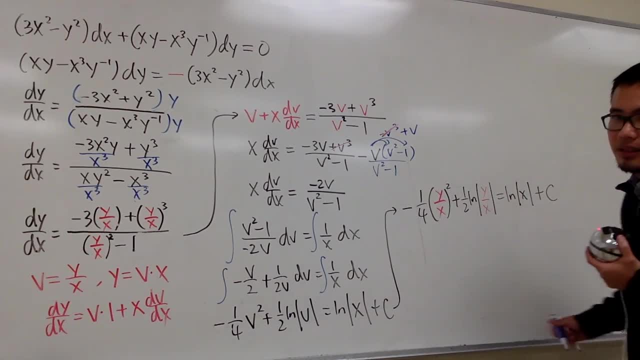 I also have to do that right here, And as long as you put this down, the test, you pretty much can get all credit, because there's no rules in the sense of how much you have to do next to simplify this answer. But I think this is pretty legit And with